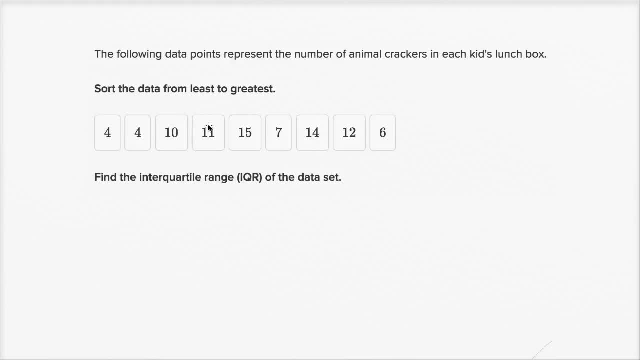 exercise. you could just drag these. you could just click and drag these numbers around to sort them. but I'll just do it by hand. So let's see: the lowest number here looks like it's a four. So I have that four and then I have another four. 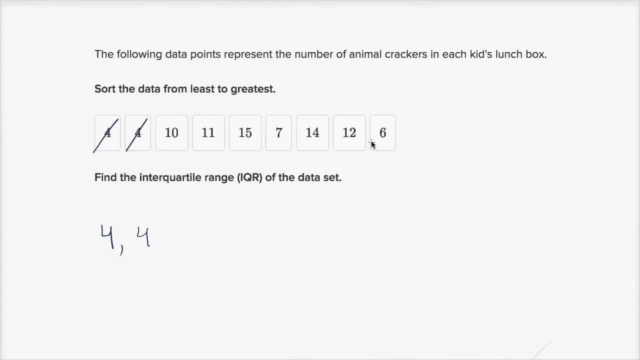 And then I have another four And let's see: are there any fives? No fives, but there is a six. So then there's a six and then there's a seven. There doesn't seem to be an eight or a nine. 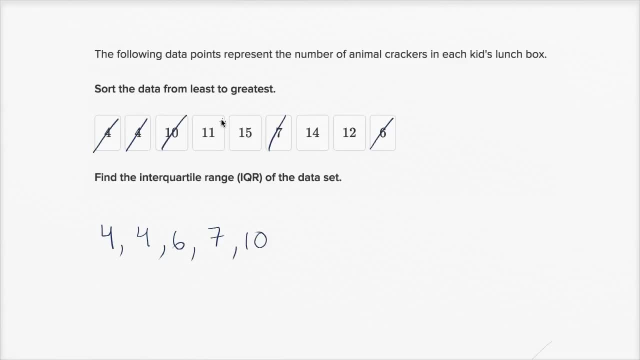 but then we get to a 10.. And then we get to 11,, 12,, no 13,- but then we get 14. And then, finally, we have a 15.. So the first thing we want to do is figure out the median here. 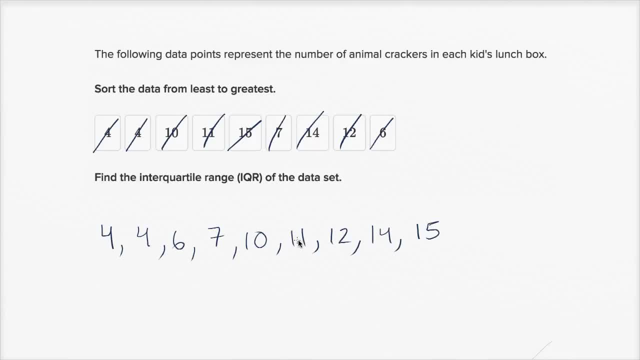 So the median's the middle number. I have one, two, three, four, five, six, seven, eight, nine numbers, so there's going to be just one middle number. I have an odd number of numbers here And it's going to be the number that has four to the left. 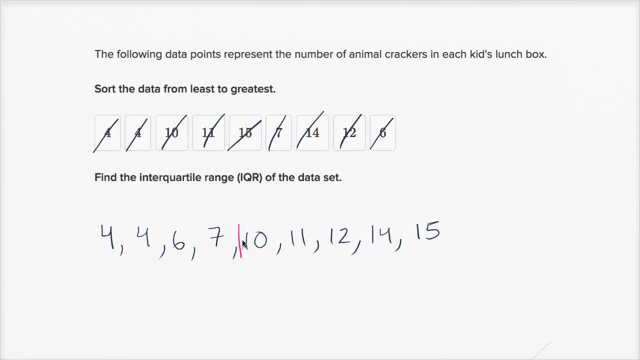 and four to the right, and that middle number, the median, is going to be 10.. Notice, I have four to the left and four to the right, And the interquartile range is all about figuring out the difference between the middle of the first half. 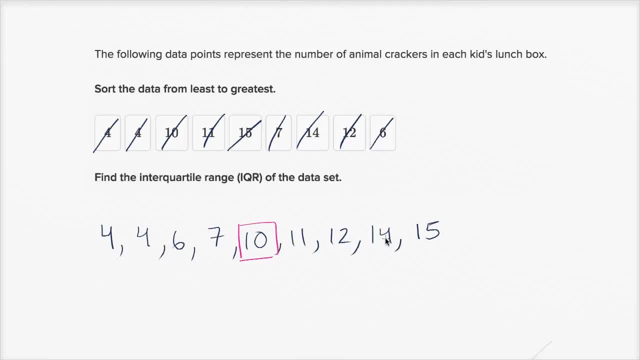 and the middle of the second half. It's a measure of spread, how far apart all of these data points are, And so let's figure out the middle of the first half. So we're going to ignore the median here and just look at these first four numbers. 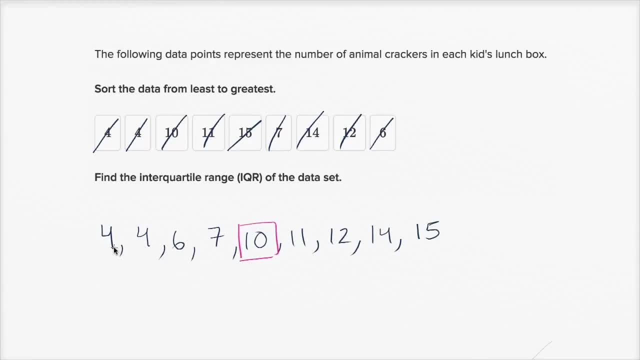 And so out of these first four numbers I have- since I have only I have- an even number of numbers- I'm going to calculate the median using the middle two numbers. So I'm going to look at the middle two numbers here. 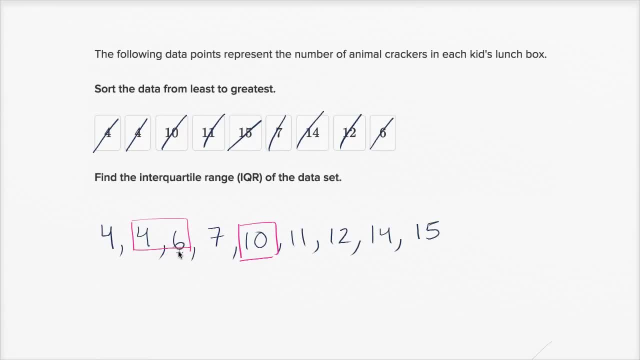 and I'm going to take their average. So the average of four and six, halfway between four and six, is five. Or you could say four plus six is four plus six is equal to 10.. But then I want to divide that by two. 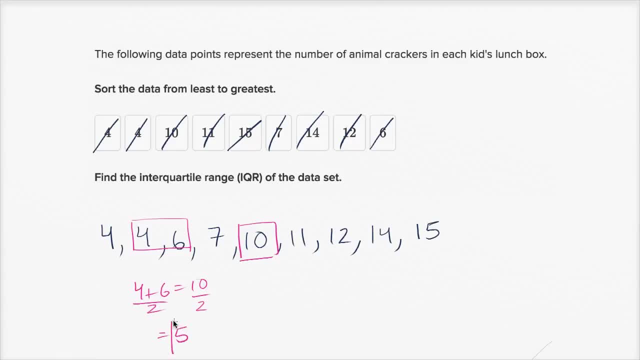 So this is going to be equal to five. So the middle of the first half is five- You can imagine it right over there- And in the middle of the second half I'm going to have to do the same thing. I have four numbers. 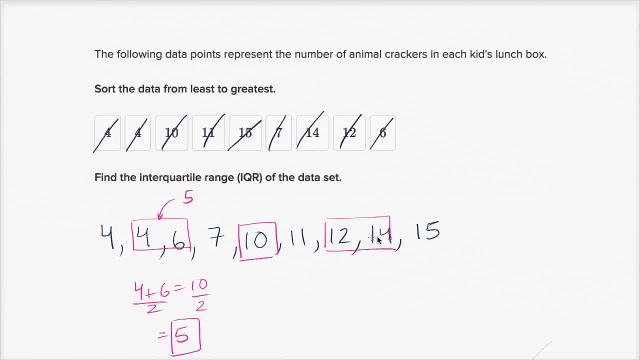 I'm going to look at the middle two numbers. The middle two numbers are 12 and 14.. The average of 12 and 14 is going to be 13.. If you took 12 plus 14 over two, that's going to be 26 over two. 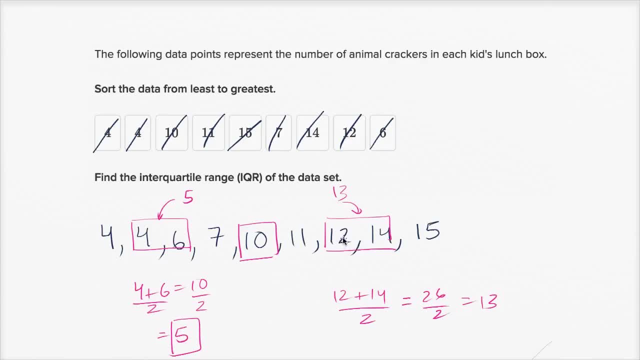 which is equal to 13.. But an easier way for numbers like this. you say, hey, like 13 is right, exactly halfway between 12 and 14.. So there you have it. I have the middle of the first half this five. 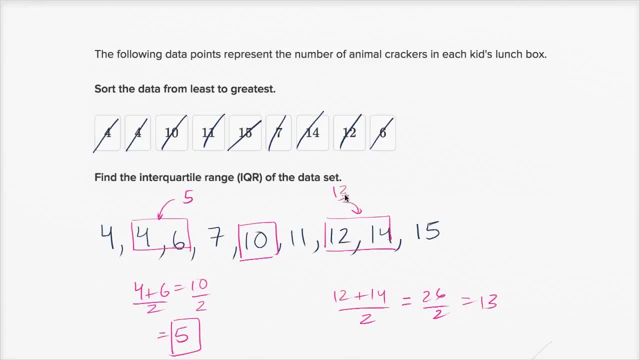 I have the middle of the second half, 13.. To calculate the interquartile range, I just have to find the difference between these two things. So the interquartile range for this first example is going to be 13 minus five. 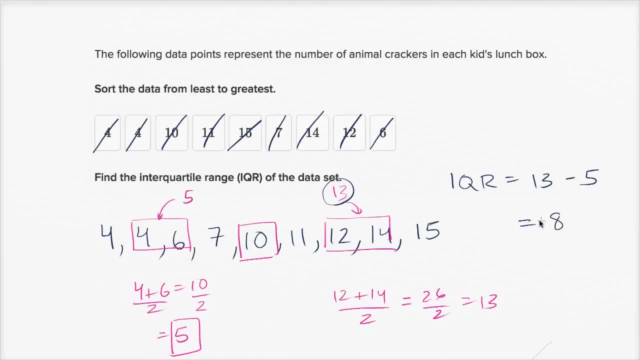 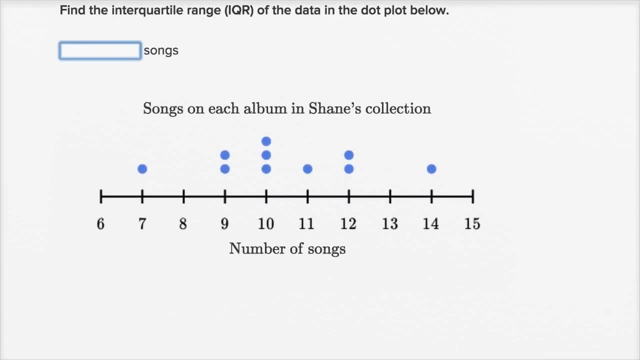 The middle of the second half minus the middle of the first half, which is going to be equal to eight. Let's do some more of these. This is strangely fun. Find the interquartile range of the data in the dot plot below. 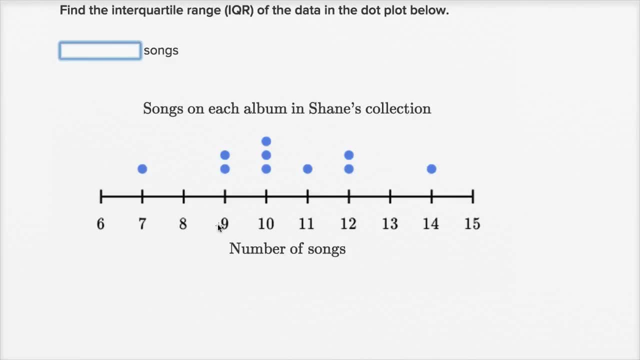 Songs on each album in Shane's collection, And so let's see what's going on here And, like always, I encourage you to take a shot at it. So this is just representing the data in a different way, but we could write this again as an ordered list. 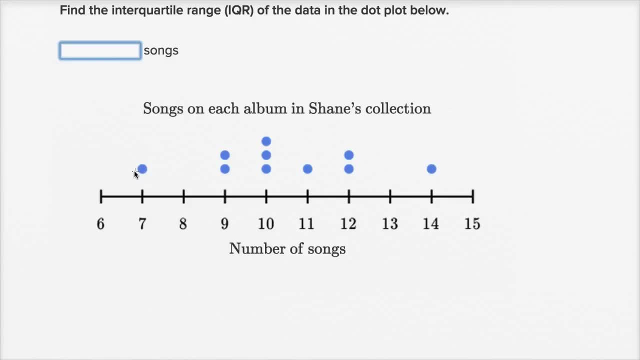 So let's do that. We have one song, or we have one album with seven songs. I guess you could say So we have a seven. We have two albums with nine songs, So we have two nines. Let me write those. 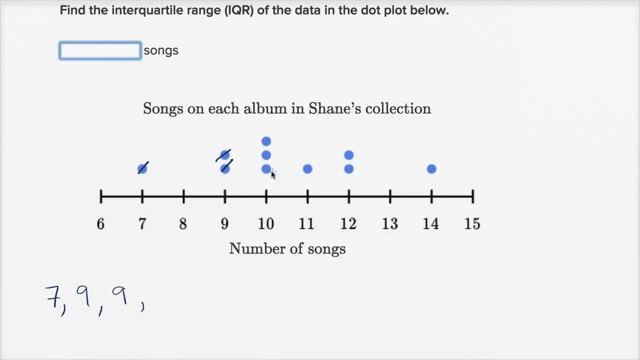 We have two nines, Then we have three 10s. Cross those out, So 10,, 10,, 10.. Then we have an 11. We have an 11.. We have two 12s, Two 12s. 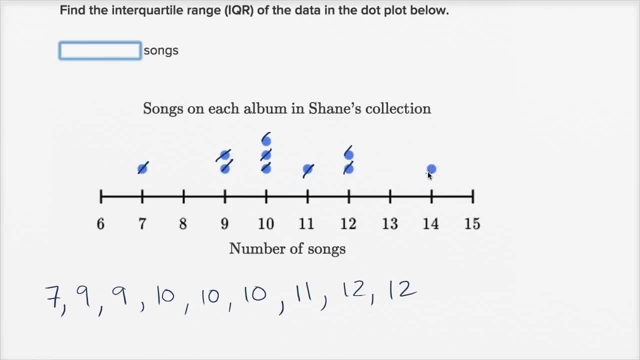 And then finally we have- so I used those already- and then we have an album with 14 songs- 14.. So all I did here is I wrote this data like this, So we could see: okay, this album has seven songs. 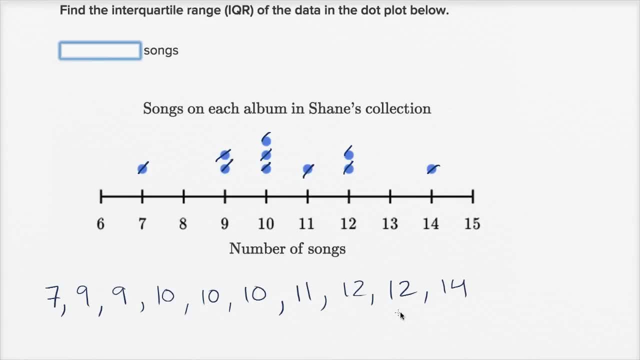 This album has nine. This album has nine And the way I wrote it it's already in order, So I can immediately start calculating the median. Let's see. I have one, two, three, four, five, six, seven, eight, nine, 10 numbers. 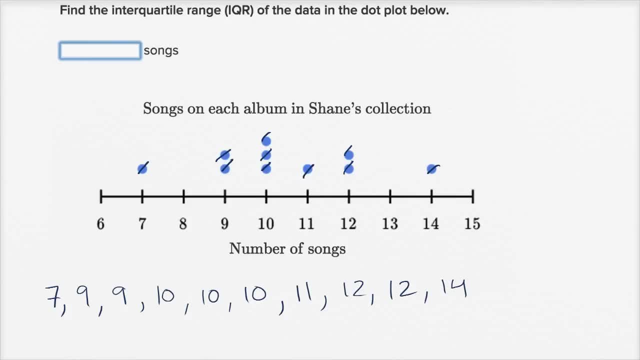 I have an even number of numbers, So to calculate the median I'm gonna have to look at the middle two numbers. So the middle two numbers look like it's these two 10s here, because I have four to the left of them and then four to the right of them. 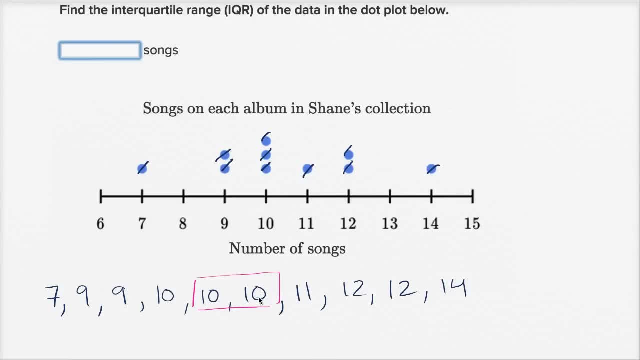 And so, since I'm calculating the median using two numbers, it's going to be halfway between them. It's going to be the average of these two numbers. Well, the average of 10 and 10 is just going to be 10.. 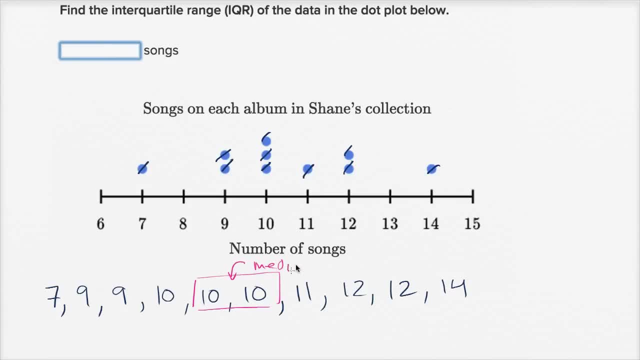 So the median is going to be 10.. Median is going to be 10.. And in a case like this, where I calculated the median using the middle two numbers, I can now include this left 10 in the first half and I can include this right 10 in the second half. 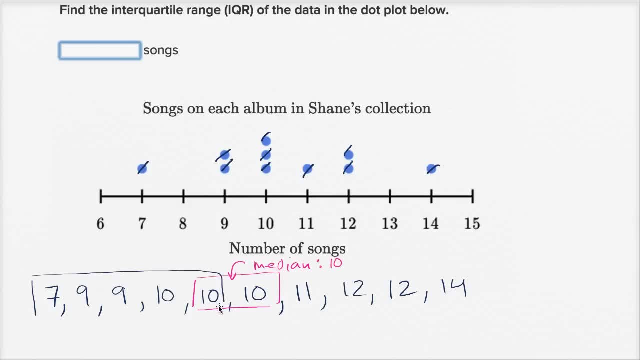 So let's do that. So the first half is going to be those five numbers and then the second half is going to be these five numbers. And it makes sense because I'm literally just looking at: first half is going to be five numbers, second half is going to be five numbers. 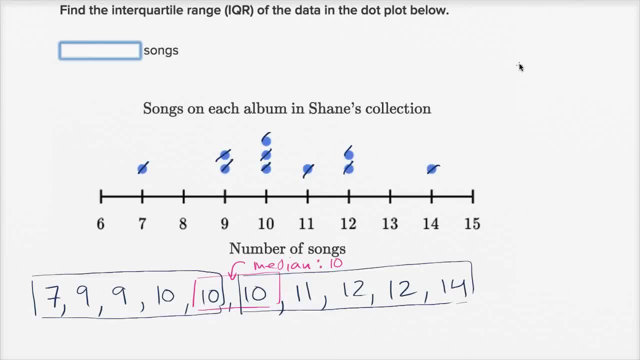 If I had a true middle number like the previous example, then we ignore that when we look at the first and second half, or at least that's the way that we're doing it in these examples. But what's the median of this first half if we look at these five numbers? 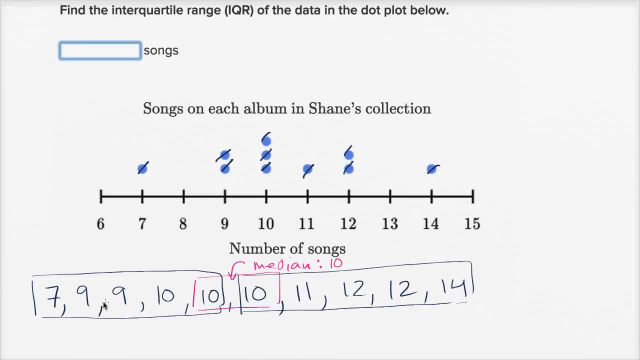 Well, if you have five numbers, if you have an odd number of numbers, you're going to have one middle number And it's going to be the one that has two on either sides. This has two to the left and it has two to the right. 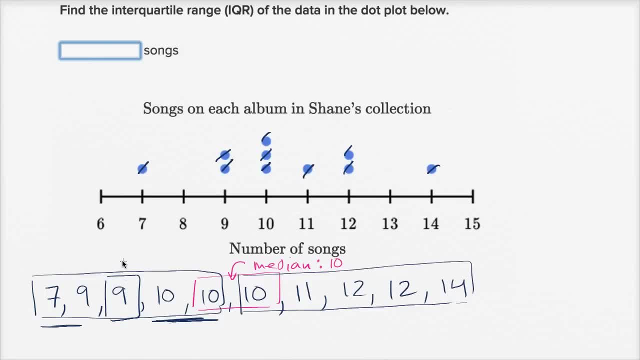 So the median of the first half, the middle of the first half is nine right over here And the middle of the second half I have one, two, three, four, five numbers And this 12 is right in the middle. 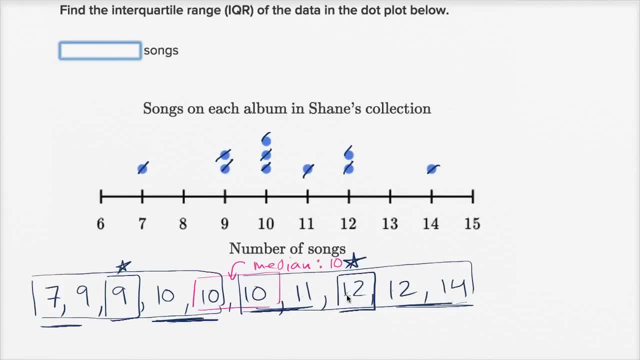 You have two to the left and two to the right, So the median of the second half is 12.. Interquartile range is just going to be the median of the second half- 12, minus the median of the first half, nine.